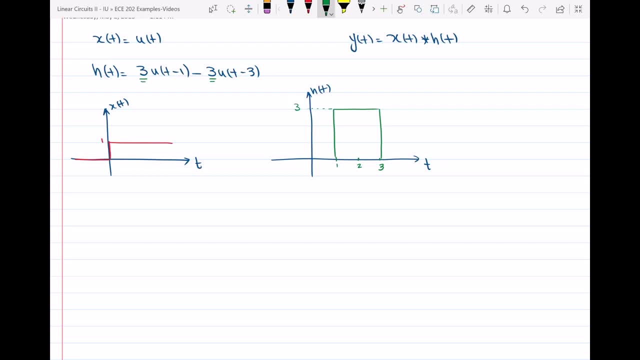 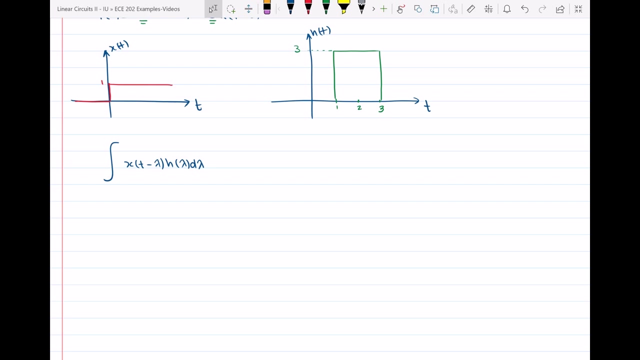 that we have over here. so now I have both signals and I know that the convolution integral is x of t minus lambda, h of lambda, d lambda. so what I have to do is I have to swap one of the functions and then shift it by T to make 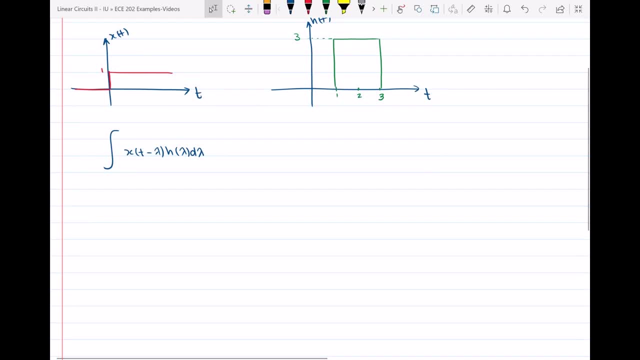 this x of t minus lambda. so what I will do is that first let's find x of negative land. so the lambda that I'm using is just a dummy variable. so X of negative lambda, because then at the end I want to use it in the next function and I'm going to close this here, because then I want to. 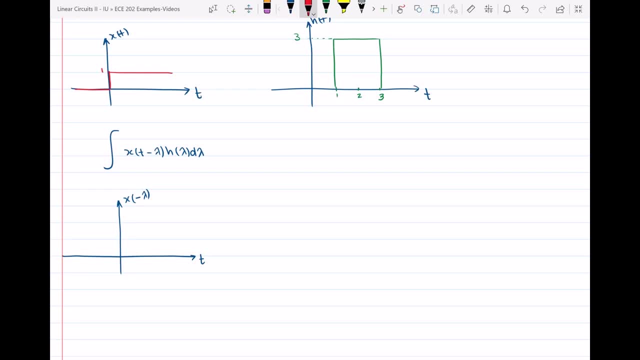 the integral with respect to t. So we have x of negative lambda. So the only thing that I did is to swap it and mirror it with respect to the y-axis, And then what I have to do? I have to shift it by t. So when I shift this function by t, my function is going to start. 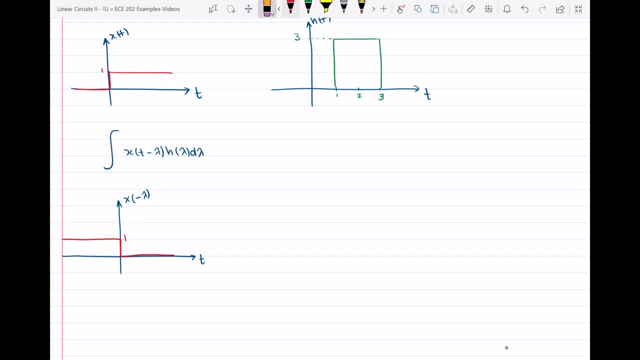 let me draw it with another color. It will be like this. So I'm shifting my function by t, So this is going to be x of actually t minus lambda. So the previous one, the red one, was x of negative lambda, And then I shifted by t so it became x of t minus. 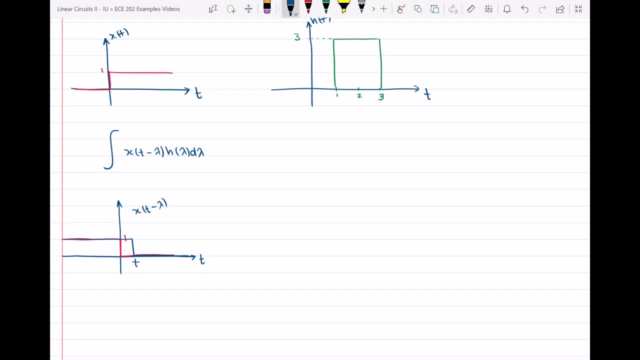 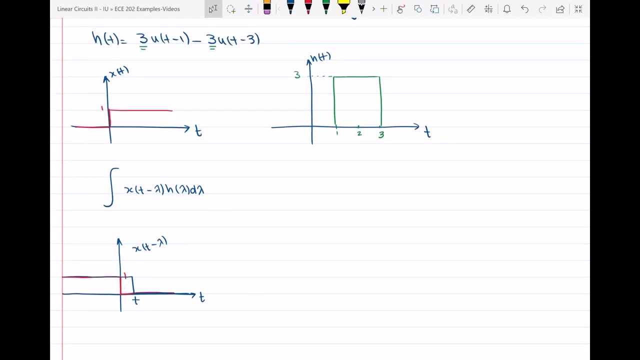 lambda. So I shifted by t, so it became x of t minus lambda, So the previous one, the lambda. Now what I have to do, I have to move my x of t minus lambda through h of t and then find the overlaps and then calculate the convolution integral. So what I'm going to do, I'm going to 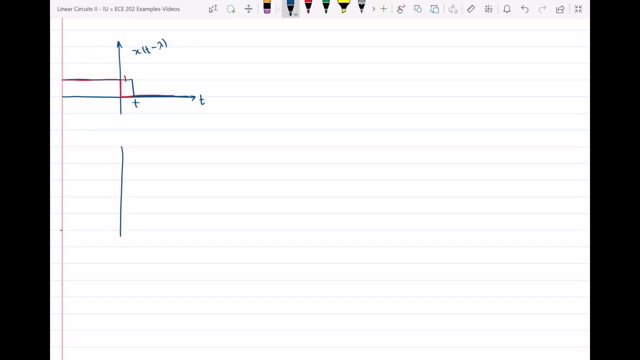 draw these two functions together in the same graph. So what I have here is x of t minus lambda, which is t over here, and then the other one was 1,, 2,, 3.. So the other one is h of t, that was over here. So this is 1,, this is 2,, this is 3.. So when t is between 0 and 1,, 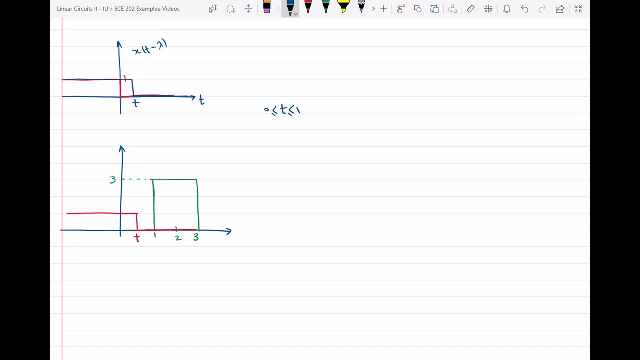 my functions x of t minus lambda and h of t or h of lambda. they do not have any overlap. So when they do not have any overlap, I can say that their convolution integral is equal to. if I call this: y of t is equal to 0. 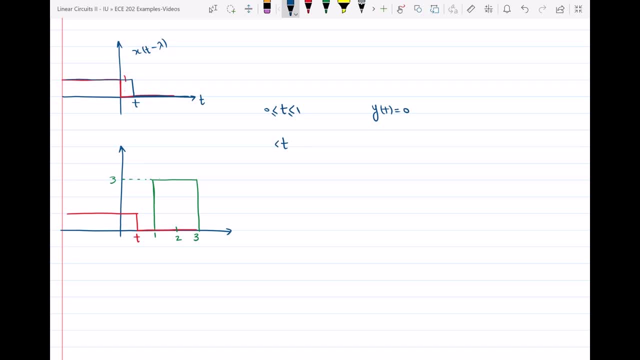 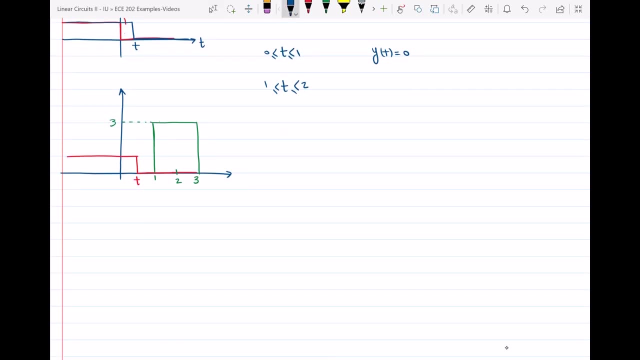 Now let's see if I move t between 1 and 2.. Let's see what will happen then. So then we are going to have again. so all the time my h of t will be at the same spot, Because h of t is not changing, it's not moving. 1,, 3, and then 2.. And now my x of t minus lambda. 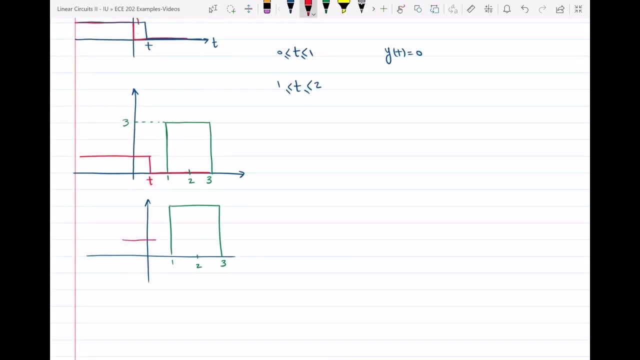 is moving so that we can have t in between 1 and 2.. Right, So this is my t. Now I have to look and see what is the interval that these two functions have overlap And then find the convolution integral or calculate the convolution integral with respect. 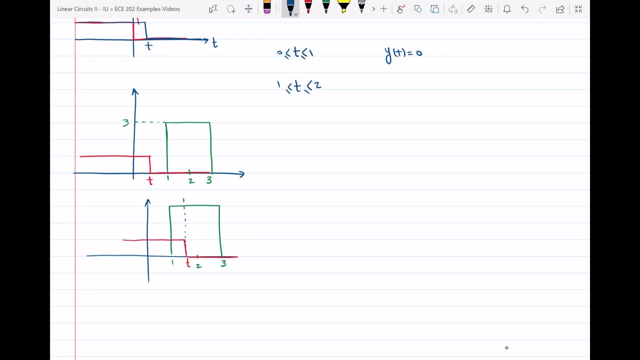 to that So clearly, from 1 to t is the interval that these two functions overlap Right. So before t, equal to 1, we only have that red function, which is my x of t minus lambda, And after t you can see that my red function, the x of t minus lambda, is equal to 0. So the only interval that I 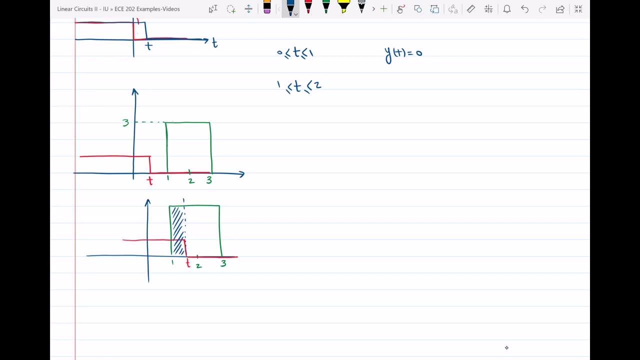 have um overlap is between 1 and t. So when t is between 1 and 2, y of t is going to be equal to integral from 1 to t. Now, x of t minus lambda, h of lambda. What is x of t minus lambda? We see that. 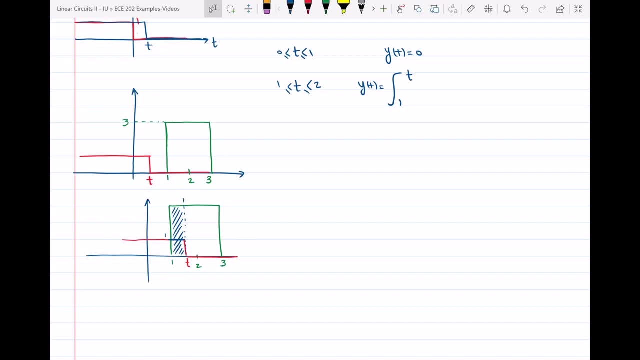 the value of this red function here is equal to 1.. And what is the value of the green function, or h of t? It's equal to 3, t lambda. So here we have 3 lambda from 1 to t, And then we're going to have 3t minus 3.. So this will be my 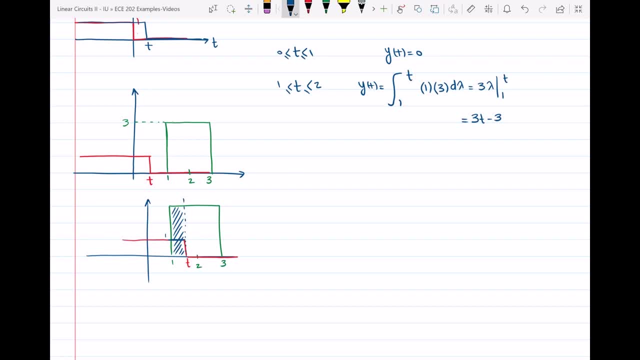 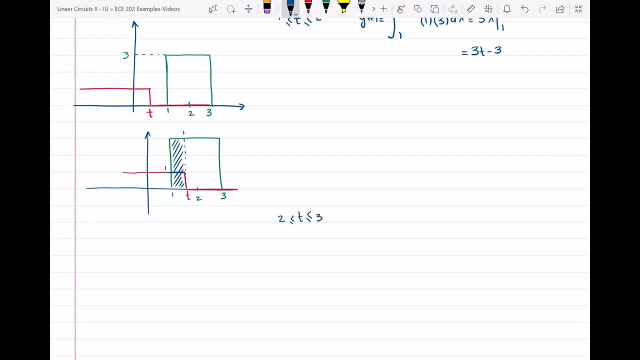 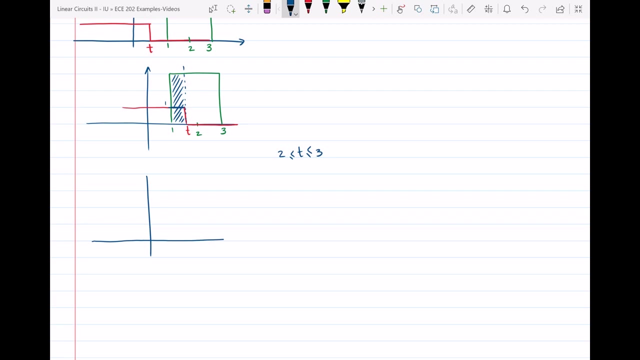 convolution when t is between 1 and 2.. Now I have to move forward. I have to move my t between 2 and 3.. So when I have t between 2 and 3, let's see what would be my t. So I have to move my t between 2 and 3.. 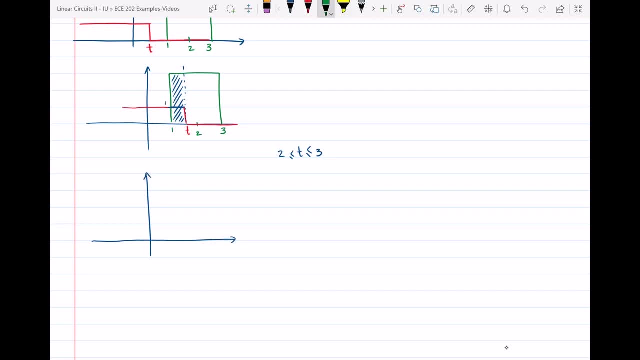 So h of t is going to be the convolution of these two functions. So h of t again, it's going to be on the same spot as it was from 1 to 3, with the height of 3.. And then x of t minus lambda will go, and then here is my 2.. 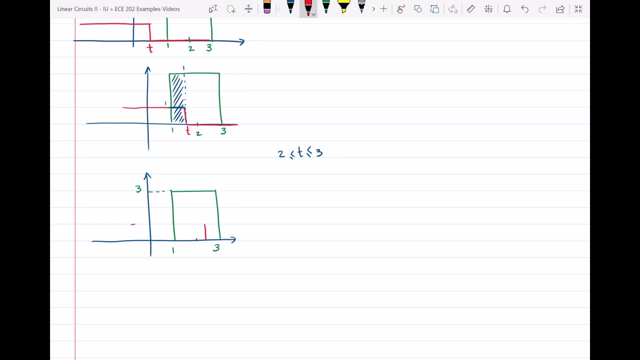 So t should be between 2 and 3.. So this will be my x of t, minus lambda Right. So t is between 2 and 3.. So again, t is between 2 and 3.. So when t is between 2 and 3,. 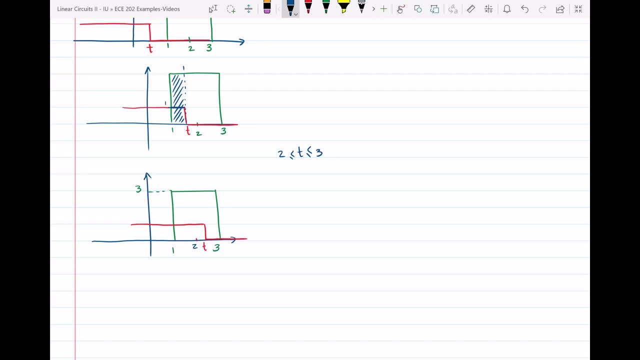 you still can see that the overlap of our functions are again between 1 and t, right? Why is this like this? Because x of t minus lambda is going to be equal to 1 all the time before time t, right. So here we again have y of t equal. the integral from 1 to t of 1 is my red function. 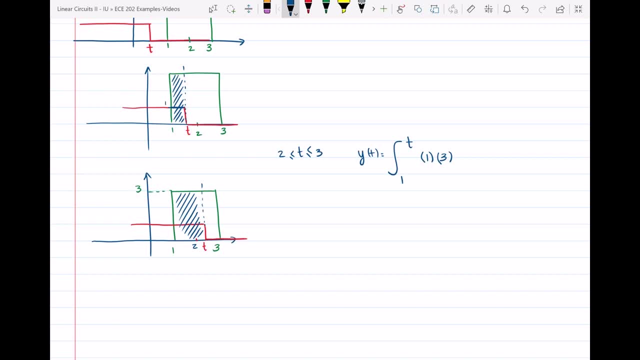 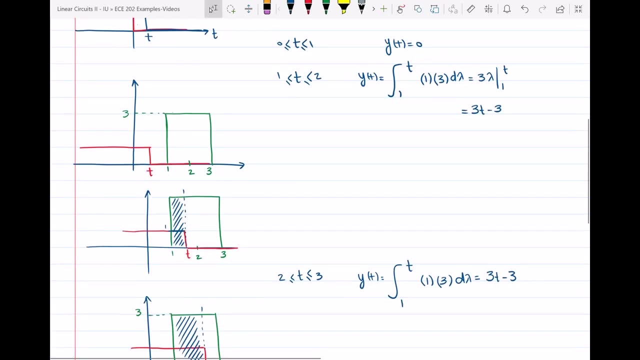 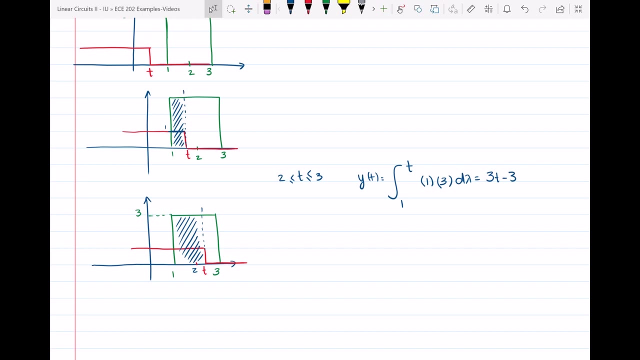 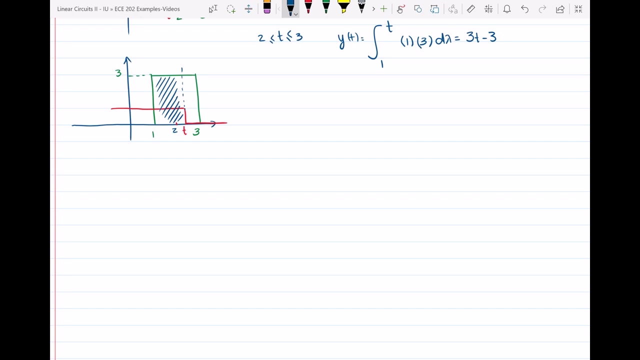 the value, and then 3 is going to be my green function, d lambda. So again we're going to have 3t minus 3, the same as the previous one. Then I have to move t between 3 and 4.. So let's do that. 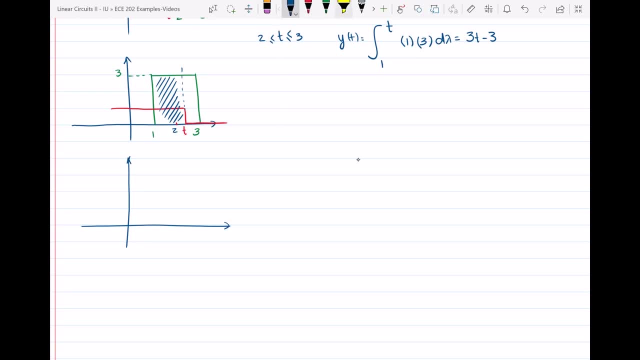 So we have t between 3 and 4.. Let me make this a little bigger. So if this is 4,, 3,, 2, and 1, then we have my red function, that t should be between 3 and 4.. 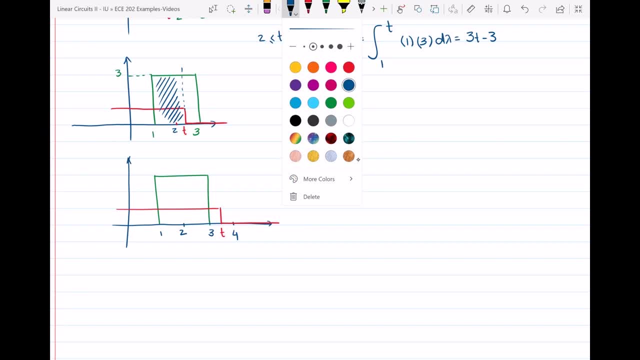 So now, here the overlap, is all this function, the green function, right? So I can say that when t is between 3 and 4, y of t is equal to 1.. So I can say that when t is between 3 and 4, y of t is equal to 1.. 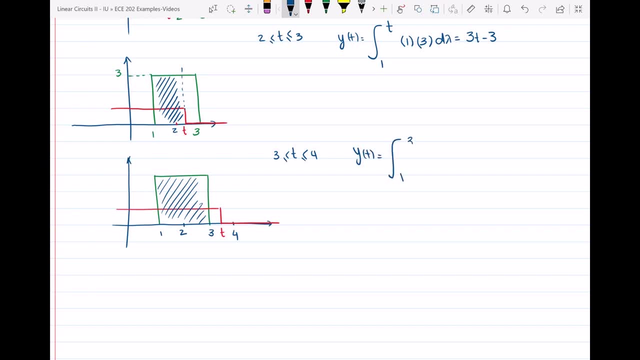 So I can say that when t is between 3 and 4, y of t is equal to 1.. So, on the other hand, t is going to be between 1, 2, 3,. the red function, the green function. 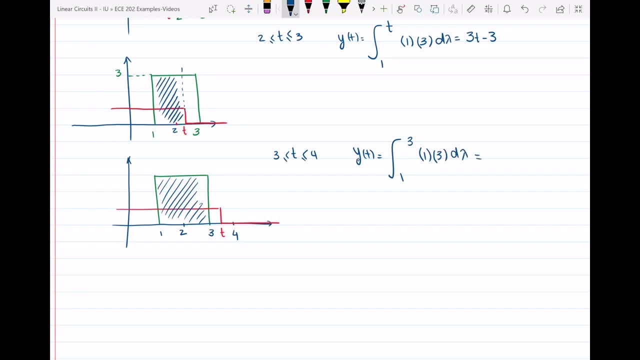 d lambda, And then we're going to have 3 lambda, from 1 to 3, which will be 9 minus 3 is equal to 6.. Now you can see that from now on, to whatever t I mean, t goes to infinity all. 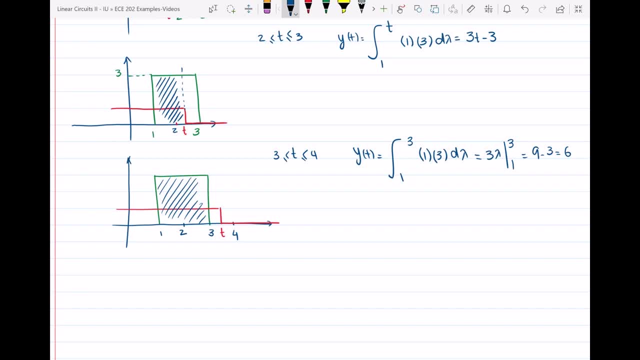 the way, If I move t to infinity, the left part of my red function will have the value t equal to 1. i mean the value of 1, right. so all the time we're going to have the same overlap from t greater than 3. so i can just delete this and say that this is true for t greater than 3. 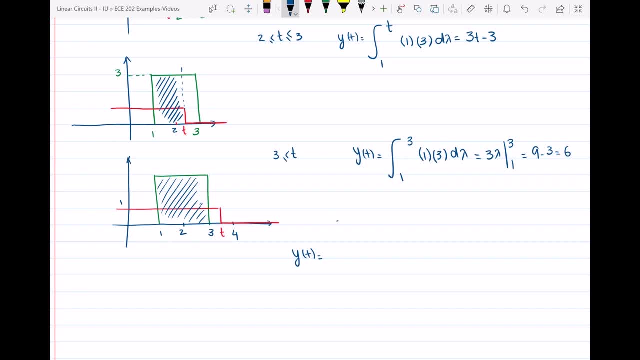 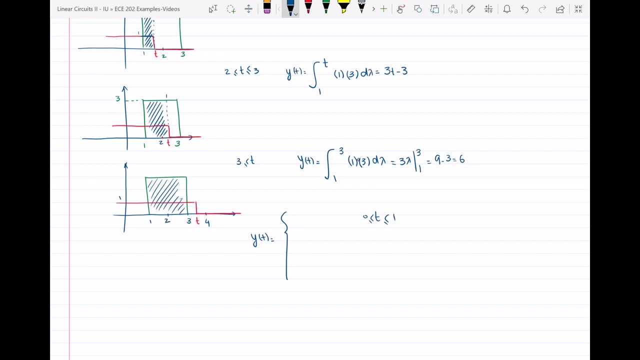 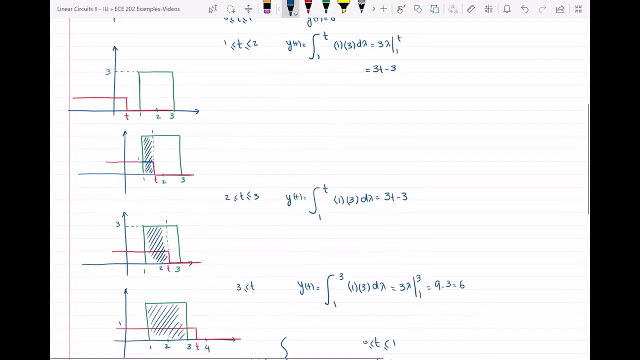 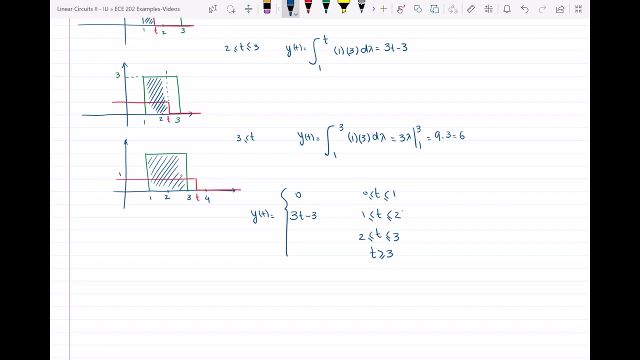 now, if i want to write my function y of t, which is the convolution of those two functions, i had t between 0 and 1, t between 1 and 2, t between 2 and 3 and t greater than 2. right now, if i go back here, we have 0. for the first one, we have 3 t minus 3. so basically for these,